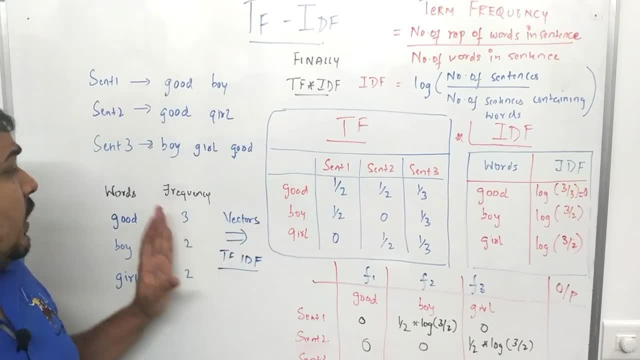 the sentences. Girl is present two times. Now. we will try to convert this whole sentences into vectors, which looks like this: you know, after applying TF-IDF technique. Now in TF-IDF, the first technique is called as term frequency. Now what does term frequency actually mean? 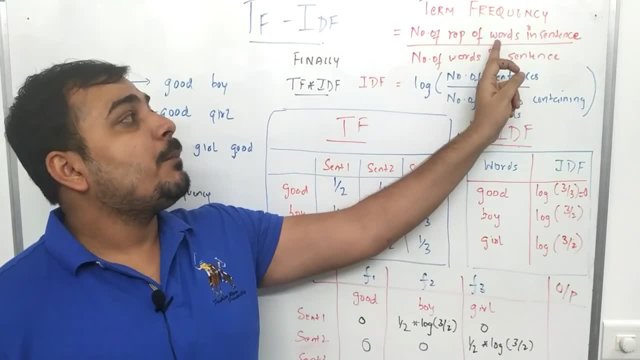 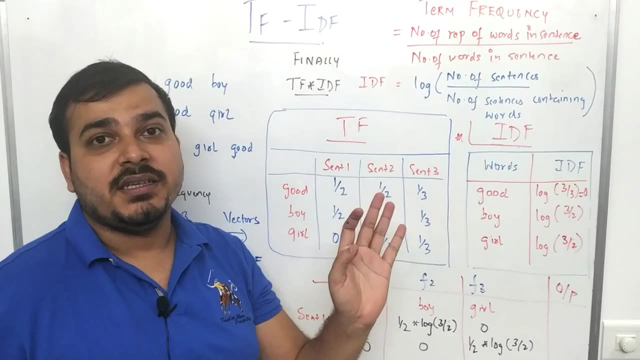 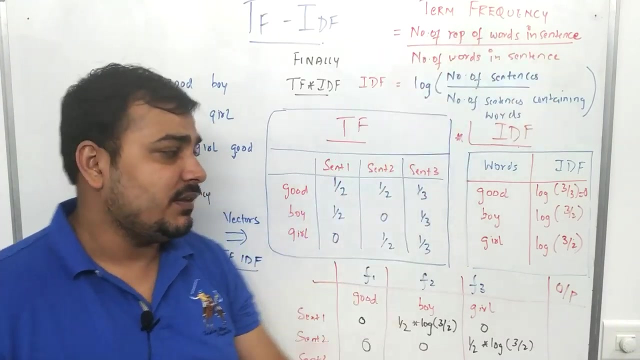 Term frequency is basically given by a formula: number of repetition of words in a sentence. number of repetition of words in a sentence- okay, only one sentence, I'm not saying sentences. number of repetition of words in a sentence divided by number of words in a sentence. Now I have these three features. I'm going. 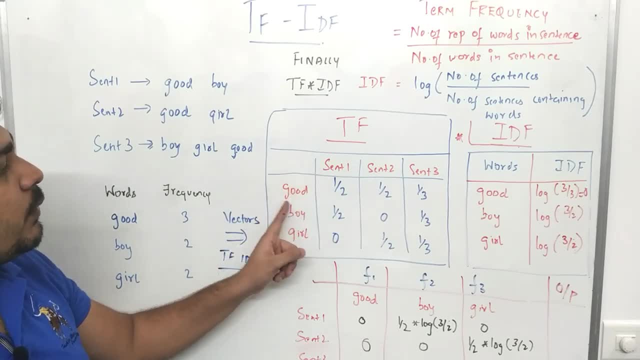 to write it over here And with respect to this, we'll try to find out the term frequency of good boy and girl in sentence one, sentence two, sentence three. Okay, Now, in sentence one I have good boy. Now, if I want to find out term frequency, number of repetition of 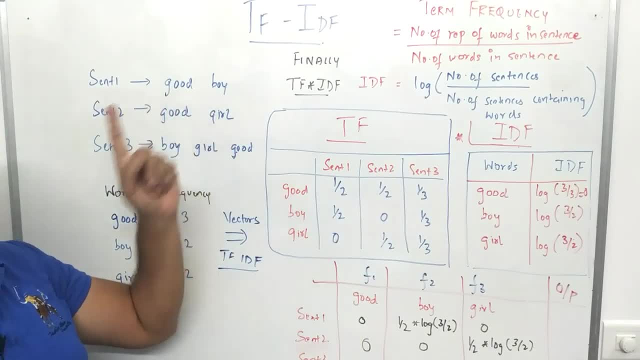 word in a sentence, right? How many times good is present over here? Only one time. One time good is present. Now, if I want to find out the term frequency, number of repetition of words is present divided by total number of words in sentence, How many words are present? 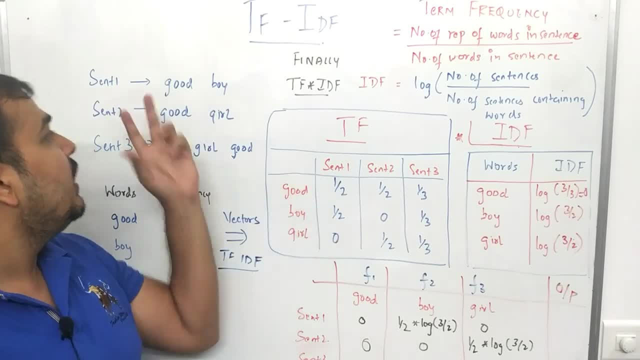 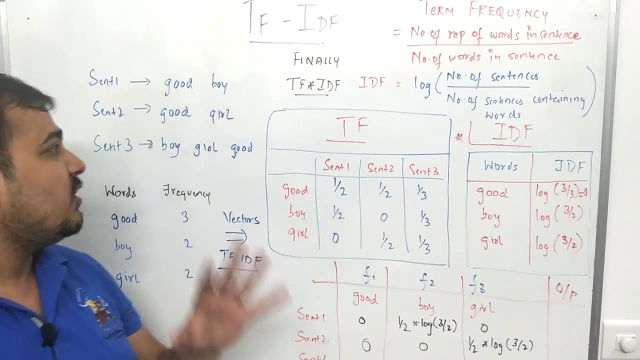 in the sentence Two, So I can write the term frequency of good in this whole corpse, in this whole corpse right, Or in this particular sentence, is basically one by two. I'll not say corpse, but we should consider sentence. okay, Is one by two. Similarly in the sentence: 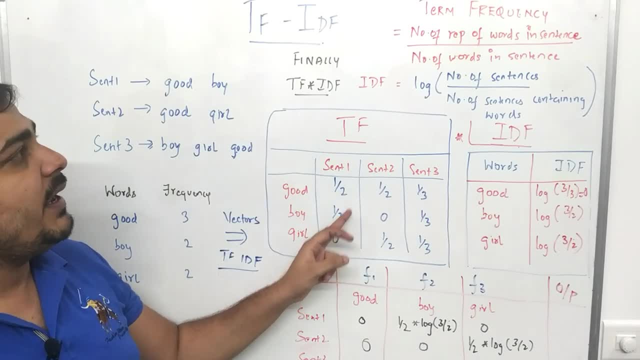 one boy is also present, right? What will be the term? frequency of boy? Again, number of repetition of words in a sentence. How many times boy is present? One Total number of words is two, One by two. Let's go and see for girl How many times girl is present. Zero times, So this will. 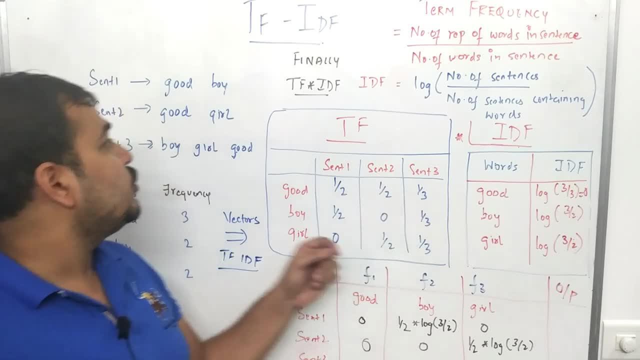 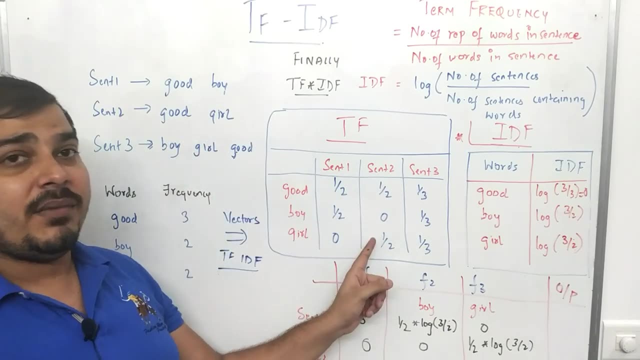 become zero right. Similarly, I'll go and compute for sentence two. In sentence two I have good and girl, So good is actually one by two, because I just have two words. Girl is one by two. Basically this is one by two. The total number of words are two. 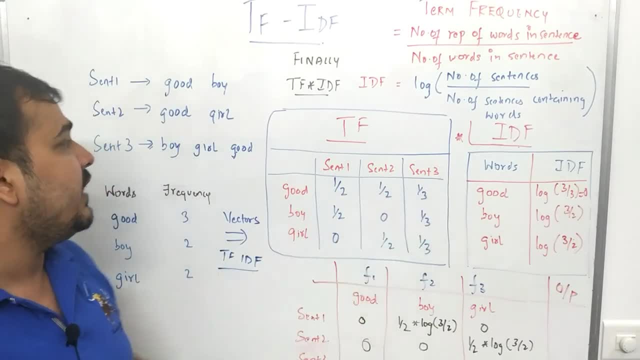 Girl. a word is actually present, one, So one by two is over here In sentence three with respect to boy, girl and good, I can just write one by three, one by three, one by three, okay, So this is how easily we actually calculate the term frequency, okay. 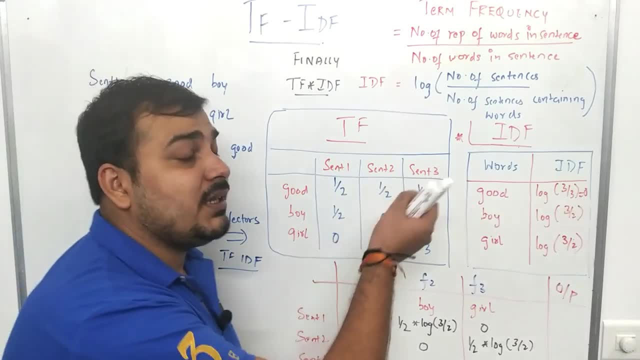 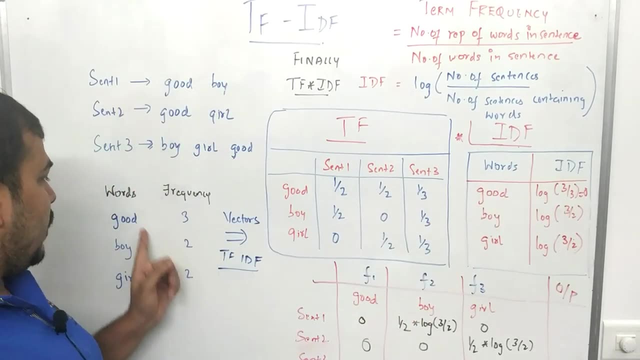 Now comes the important thing that is called as inverse document frequency. okay, Now, inverse document frequency. I'll again take the words, all these particular words, good boy and girl, and then I'll try to calculate the inverse document frequency. Now, inverse. 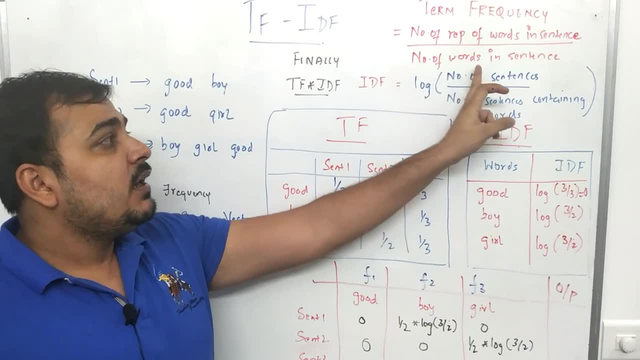 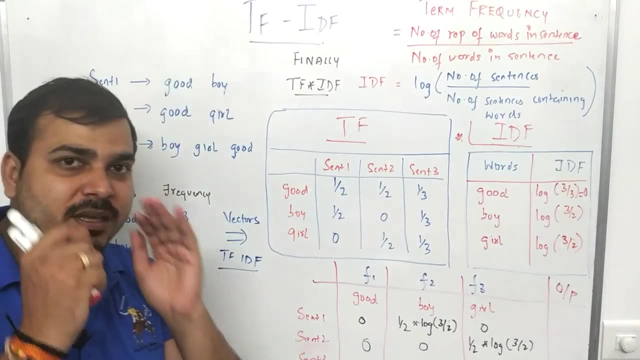 document. frequency basically says log of right number of sentences. Understand how many number of sentences are there? Three In every situation. for every word, the number of sentences will be three. It will be fixed Divided by number of sentences containing. 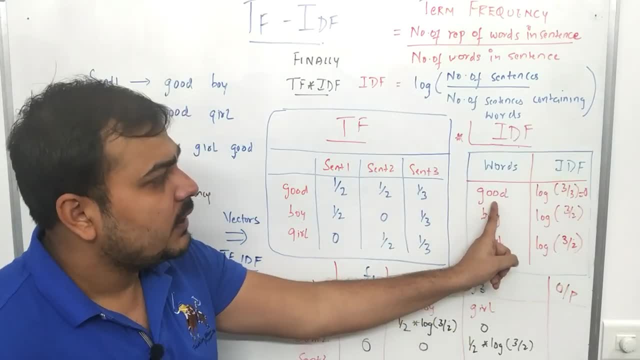 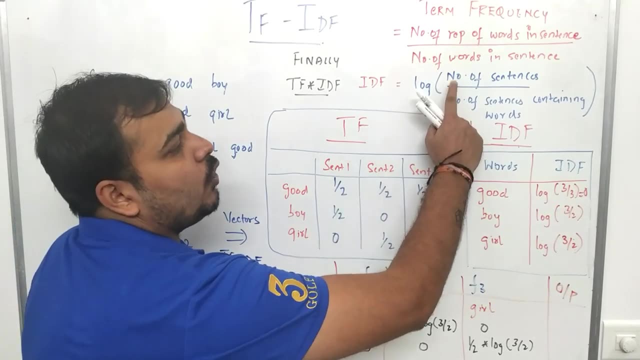 the word. Okay, Now if I want to compute for sent good in sentence, one right, And suppose I want to calculate the inverse document frequency for good, First of all we'll go and write log of how many number of sentences are there? Three Right, So I've written three Then. 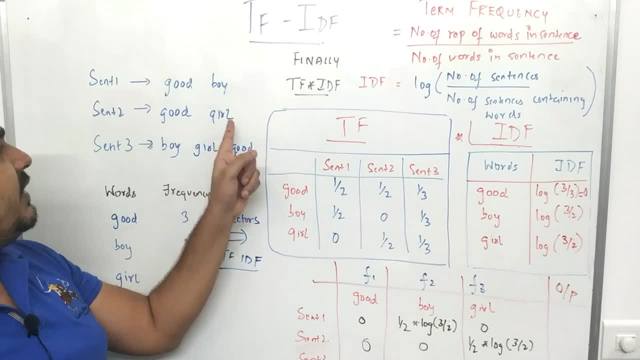 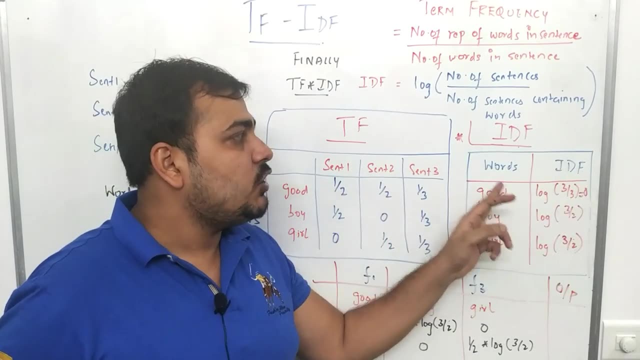 how many sentences contain this word good? You see over here, good is present here, here here. So the count will be three. So log three by three is nothing but zero. If I want to find out the inverse document frequency, I'm basically using this formula. I'm getting. 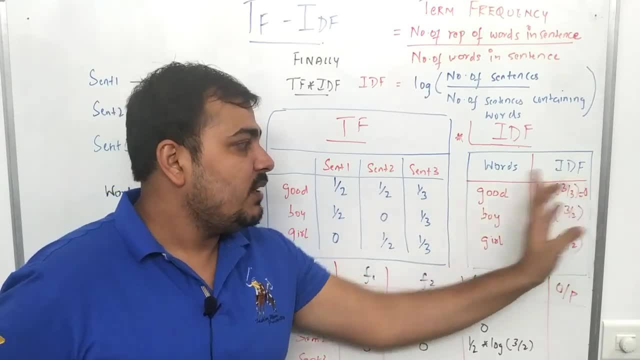 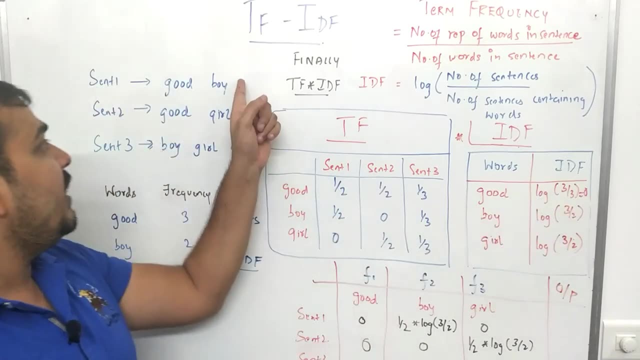 the value as zero for good, And remember this value will be zero itself. Now, with respect to the second word, boy. how many number of sentences are there? Log of three, Okay, fine. How many times boys are present? Boy is present? One and two In sentence one. 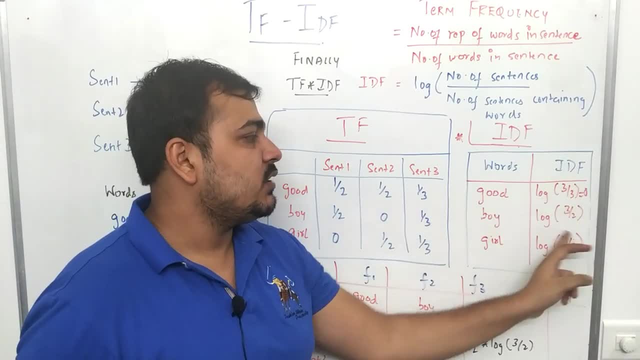 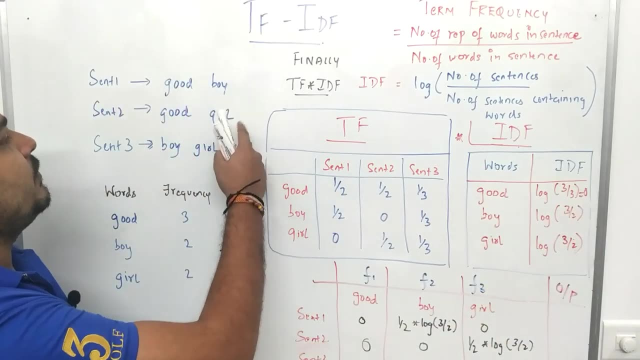 and sentence three. So log of three by two, Right, So this is my inverse document frequency for boy word. Now inverse document frequency for girl word is again log three by two, because two times girl is present. Okay, And the total number of sentences is three. Right, I have? 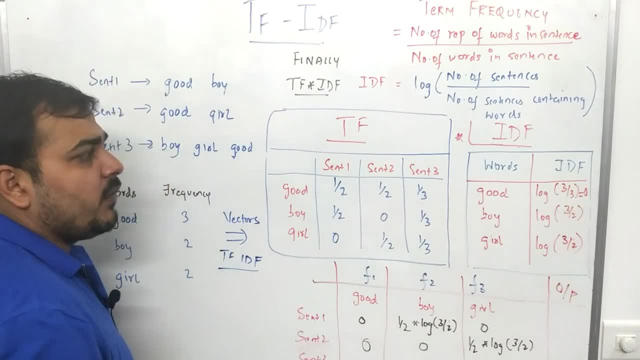 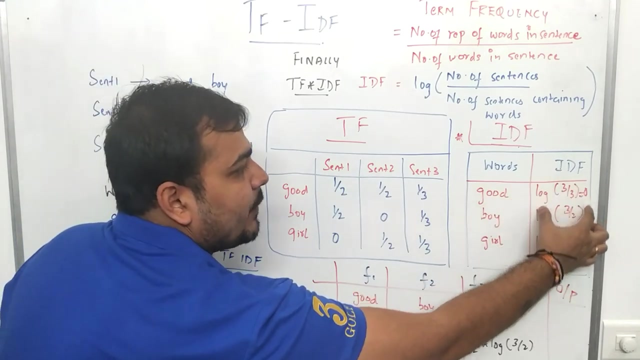 got this inverse document frequency Pretty much easy. Now what is my final goal? I have to multiply: term frequency multiplied by inverse document frequency. So what I'm going to do, I'm going to take this good boy and girl. These are my features. Now, with respect to sentence one, I have to multiply. 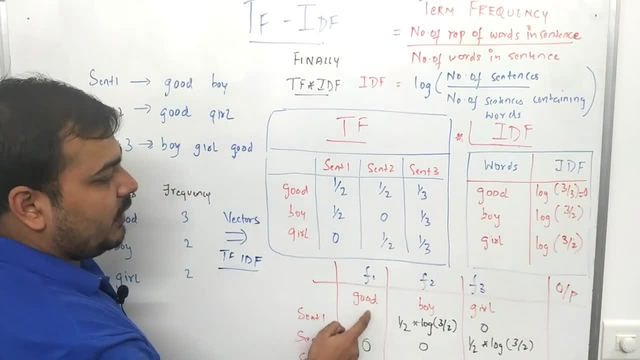 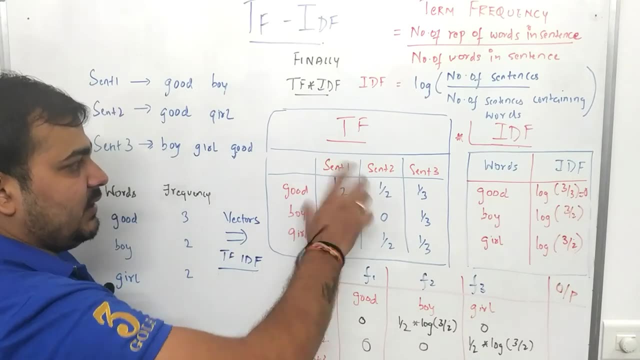 with this, With these values, So in f1,. good, that is over here, and this is my feature one Right In sentence one. Again, I'm taking sentence one. I'm just traversing this like this: Sentence one is coming here and good boy girl is coming over here, I'm taking 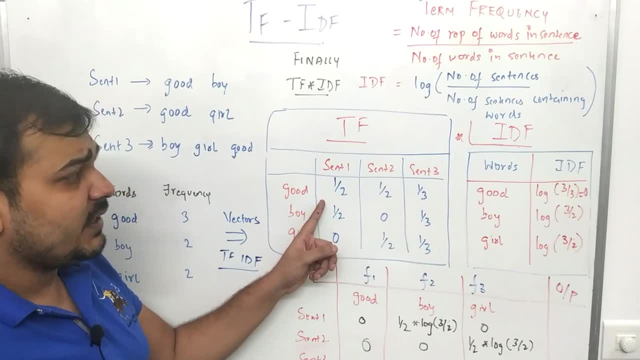 sentence one. I'm taking sentence one, I'm just traversing this like this: Sentence one is coming here and good boy girl is coming over here. Okay, So I have to write this as Now, with respect to sentence 1, I will be multiplying this value with this, this value. 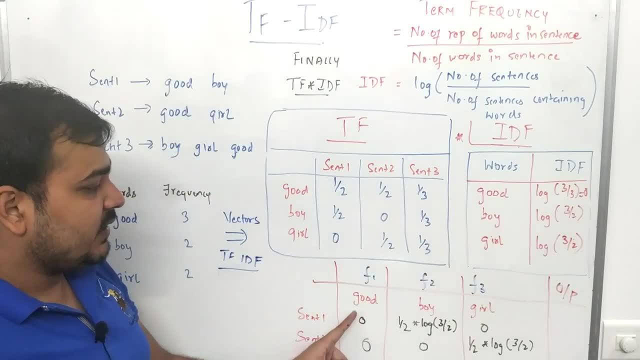 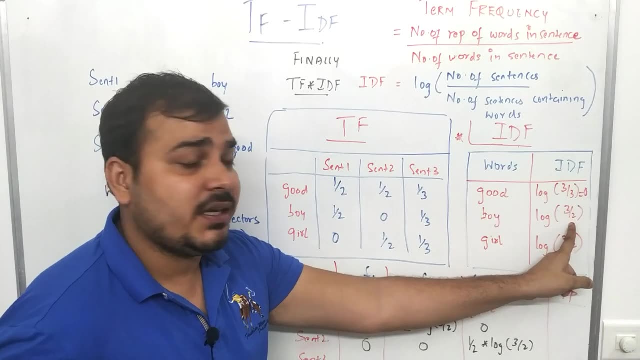 with this, this value with this. So in feature 1 you can see good, 1 by 2 multiplied by 0 is nothing but 0. With respect to y, 1 by 2 multiplied by log of 3 by 2.. 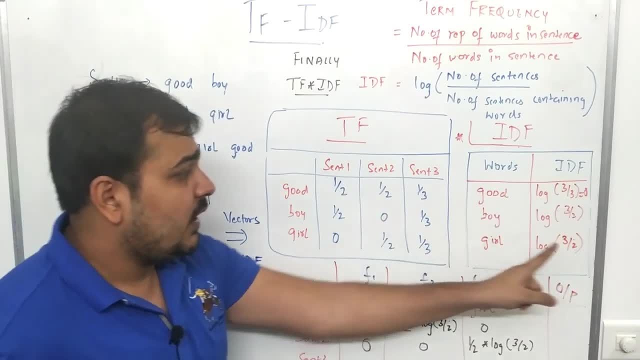 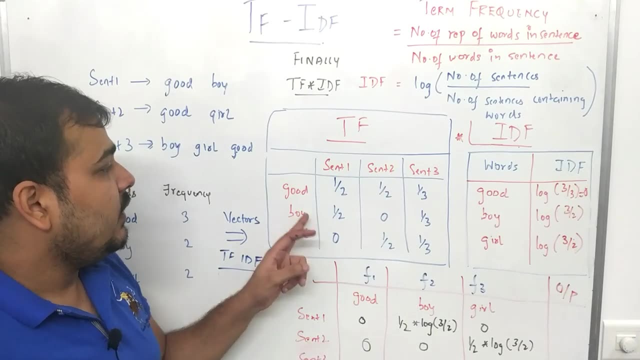 So here I am getting this value. In case of girl, this is 0, so I, multiplied by this is nothing but 0.. Now, similarly, with respect to sentence 2, you can see over here again sentence 2, over here: 1 by 2 multiplied by 0 is again 0, 0. multiplied by log of 3 by 2 is again 0, 1. 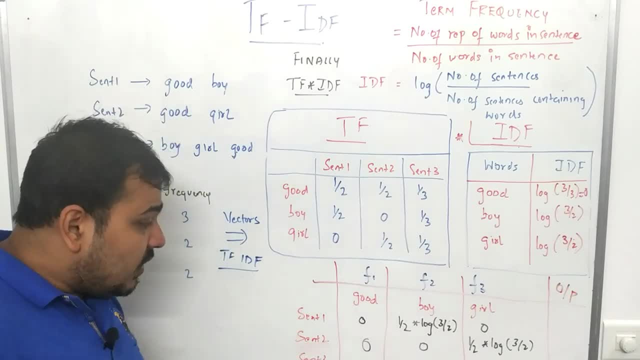 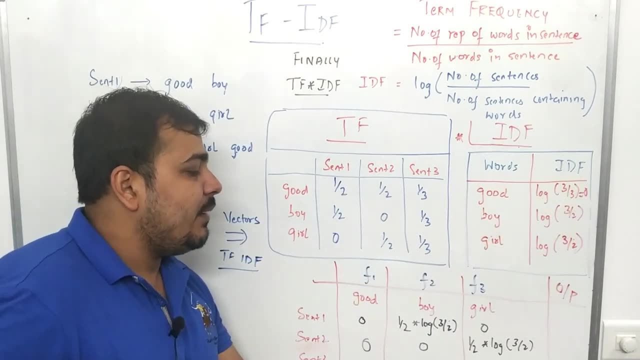 by 2 multiplied by log 3 by 2, is this value? Now in the third sentence, first word again: 1 by 3 multiplied by 0 is 0,. 1 by 3 multiplied by log 3 by 2, 1 by 3 multiplied by log 3 by 2, 1 by 3 multiplied by log 3 by 2.. 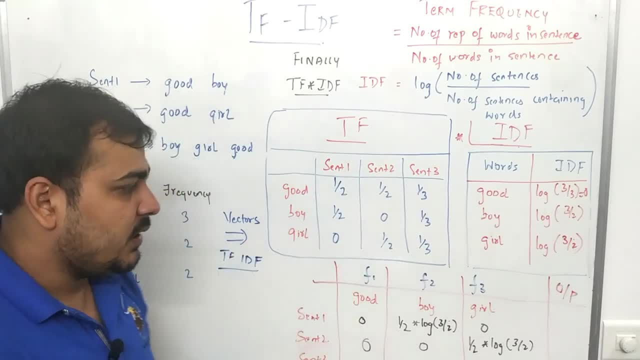 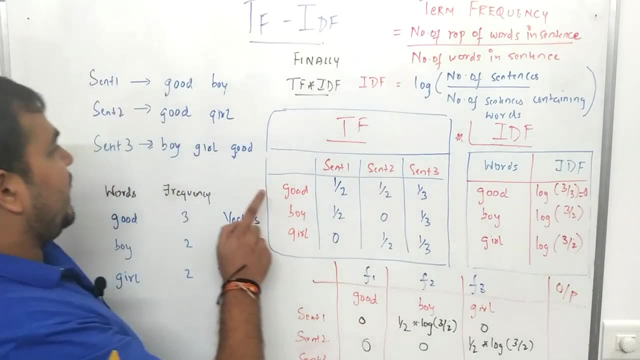 So these two values are. come Now. understand most important thing, guys. When we are using bag of words, we just have values like 1s and 0s. But just understand, In the first sentence, where I have good boy right over here, the importance is basically: 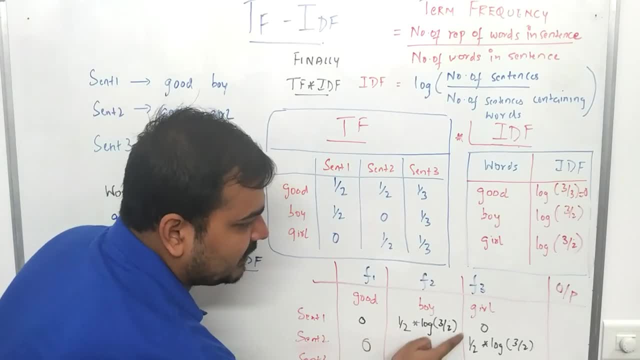 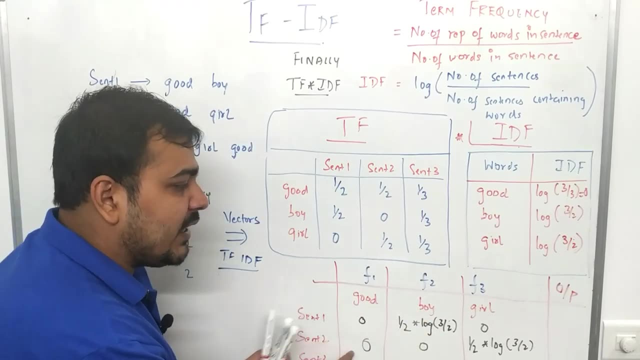 given to the boy. You can see by this because this value is coming as higher when compared to the other values in the future. Right, we are saying something about the boy Now, with respect to sentence 2 also, you can see, good girl. 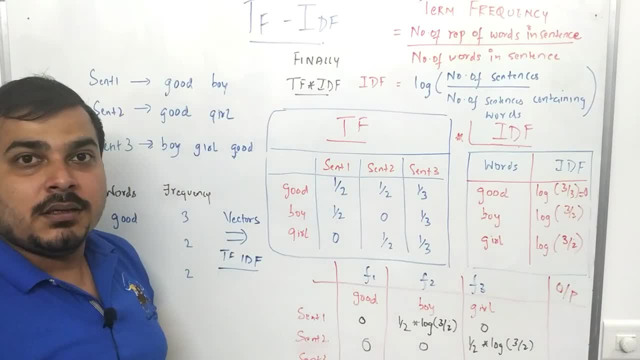 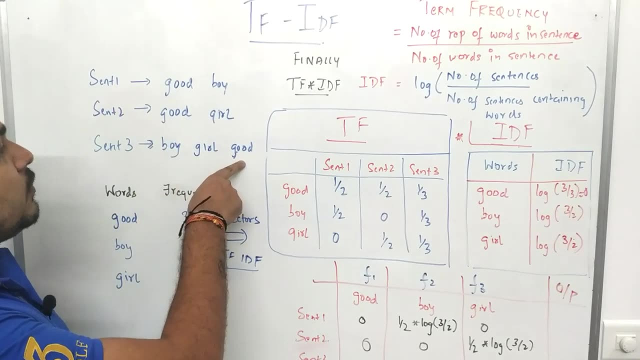 Good is not given that importance, but girl is definitely given this particular importance. You know, there is some semantic meaning. We are trying to bring some semantic meaning In the third sentence also. again, you can see, Because this good is present frequently in every sentences, right? 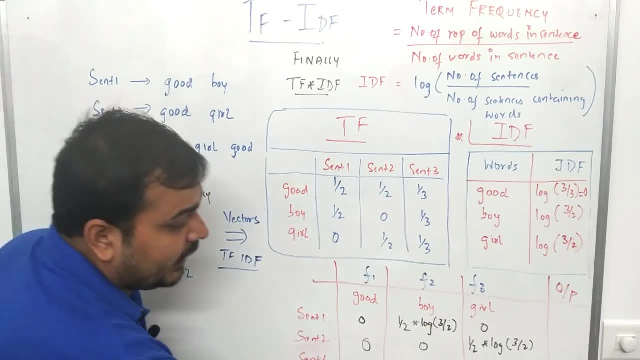 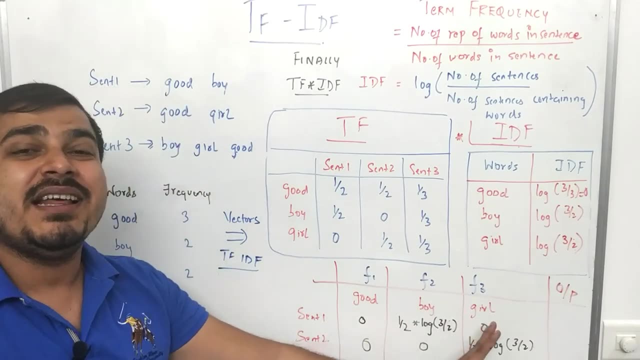 It may have the same meaning. What about boy and girl? Now, here see again. boy and girl are given the more importance. Now just try to compute these values and you will be getting a different, different values. You will not just be getting 1s and 0s. 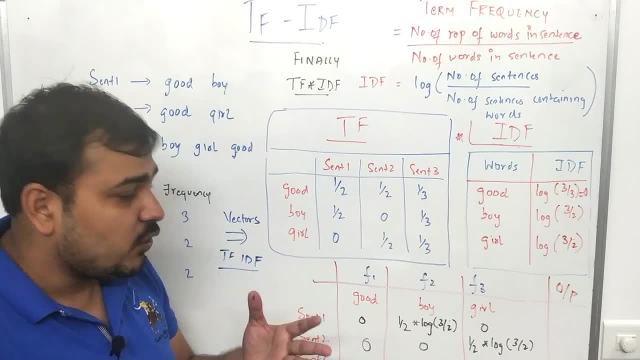 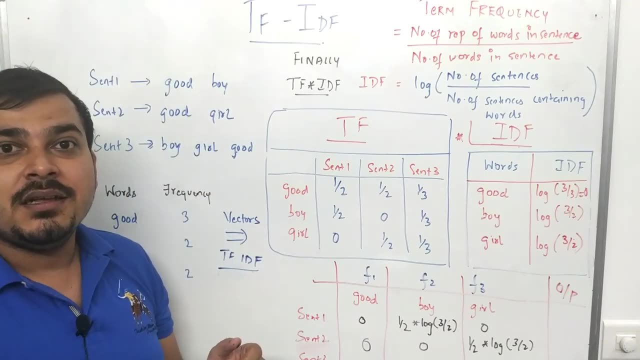 Here you will be getting in decimals like 0.17, 0.37, 0.47.. Now this is just with the example of 3 sentences, guys. Just again a simple example. Just imagine, when you have huge number of sentences at that time, how this particular 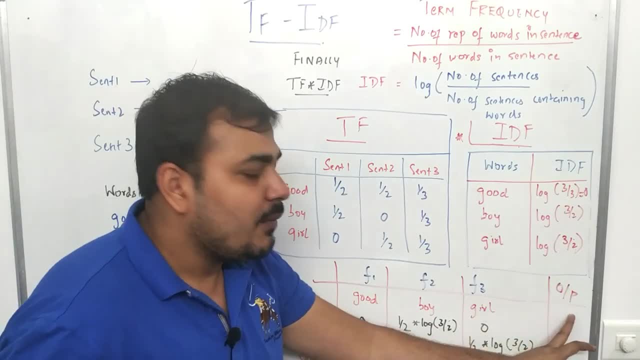 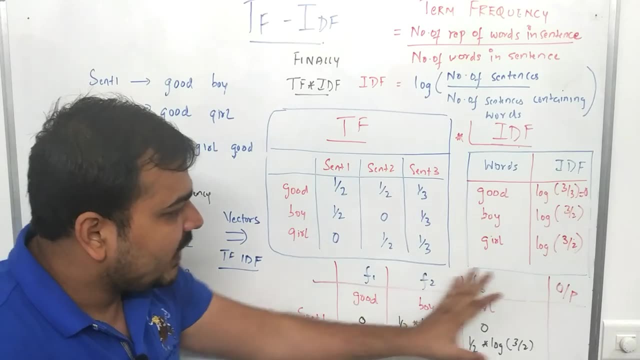 thing will work. It will work in a wonderful manner, right And always remember I will be having an output feature. This will be my dependent feature. Now, after I convert, this is basically my vectors with respect to the sentences. Now I will take this independent feature, give it to my model for training. 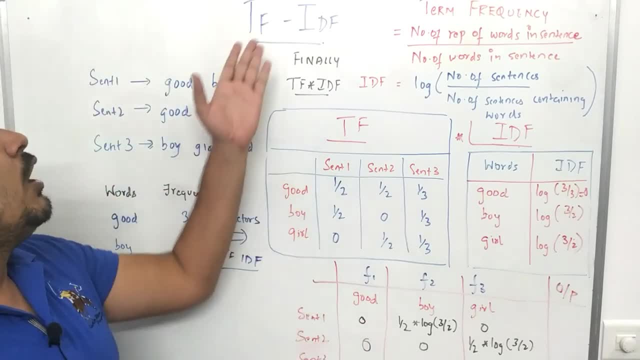 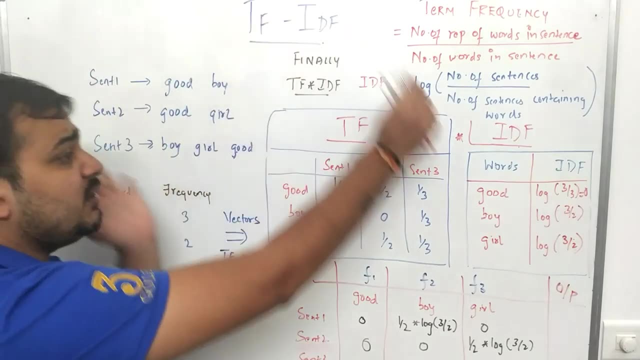 This output will be treated as a dependent feature And this is how we actually compute TFIDF, that is, term frequency and inverse document frequency. So I hope you like this particular video. I hope you have understood this strategy. Please make sure that you refer again and again.